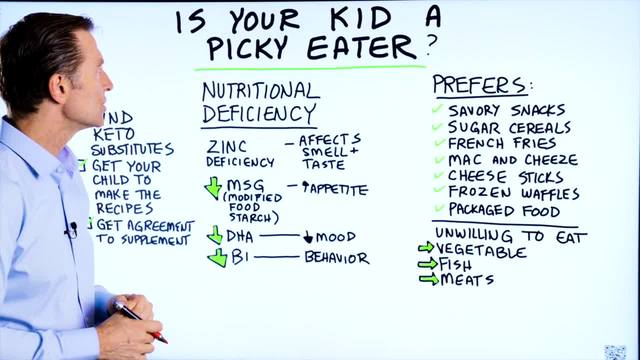 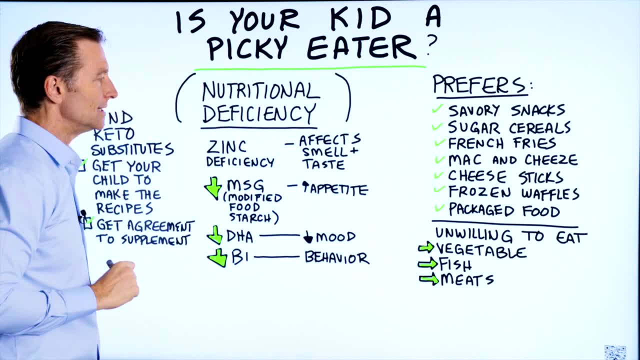 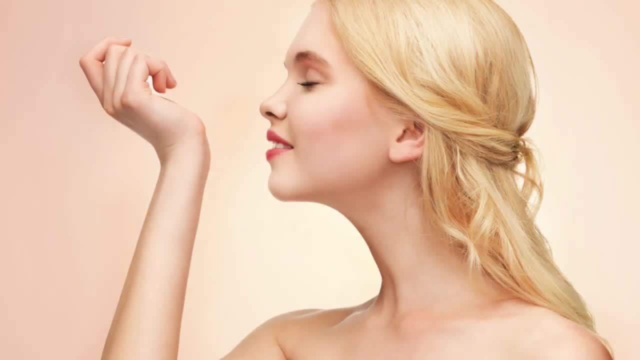 it's very, very difficult to get your child to consume the right types of foods. But let's talk about what nutritional deficiency we're dealing with. The main one is a zinc deficiency. You see, zinc affects smell and taste, And the other problem is if you're consuming these foods. 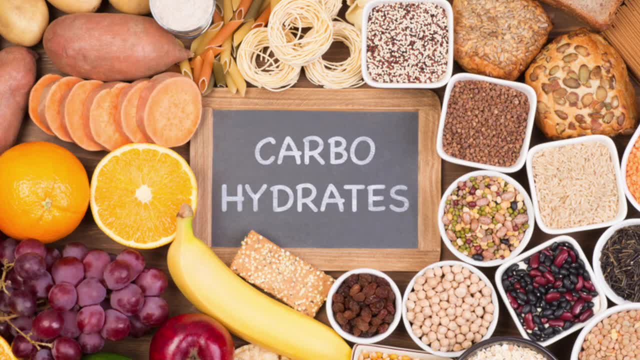 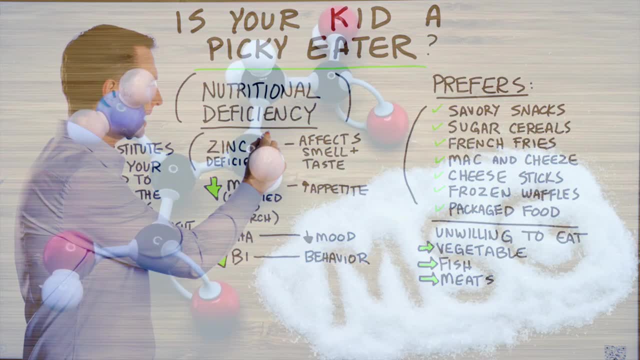 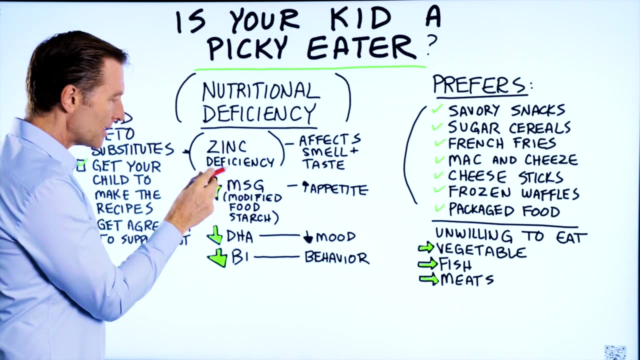 you're going to create a zinc deficiency, And if you're consuming refined carbohydrates or sugar, you're going to create a zinc deficiency. So this is number one: You want to put the zinc back in Two MSG. There are so many of these types of foods that have either MSG, monosodium glutamate. 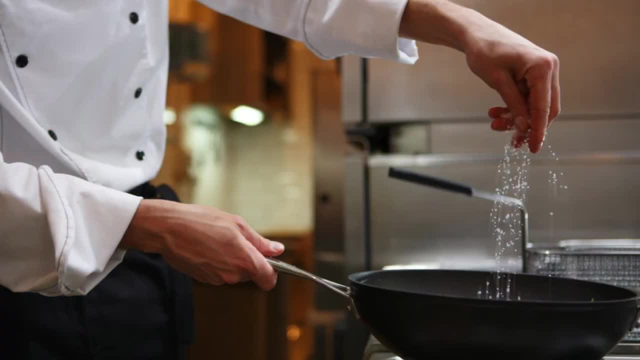 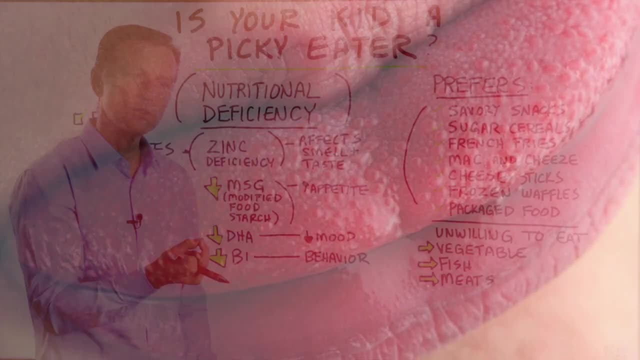 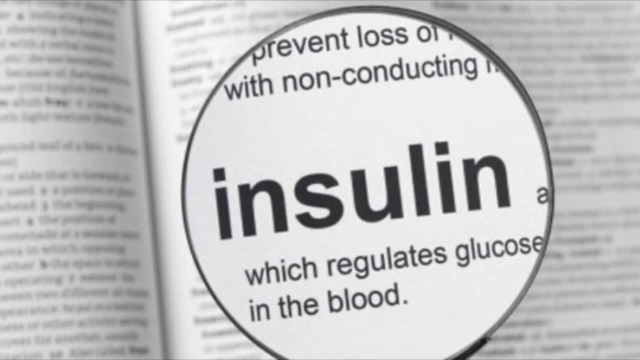 or modified food starch, Because this ingredient causes that savory sensation, It dilates the taste buds, It makes the food taste better than it really is And also it'll retain water and it will increase appetite and it increases insulin. It's not good and you want to make sure that you read the labels and 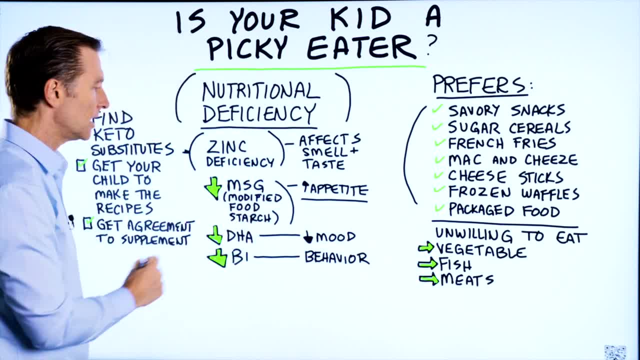 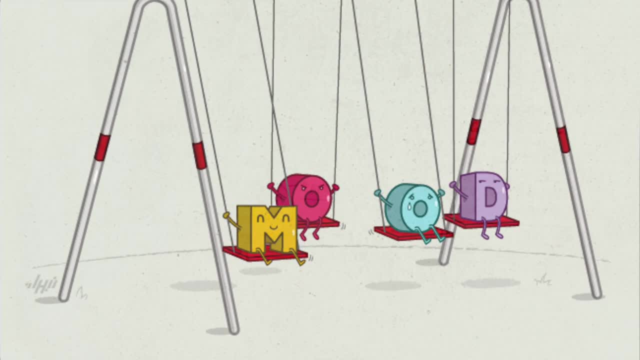 make sure your children do not consume anything with MSG or modified food starch, And also a lot of this is in fast food restaurants. Now, if the child is lacking DHA, which they usually are, that can affect the mood, especially anger, as in trying to get your child, 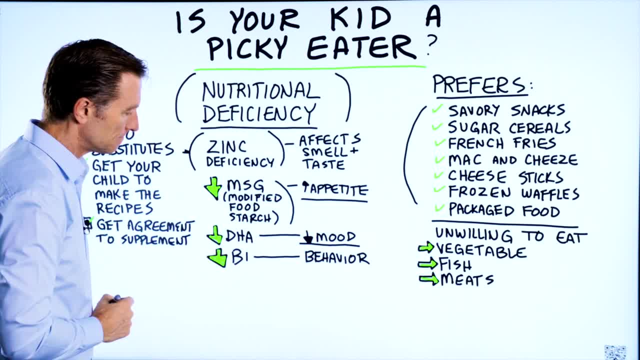 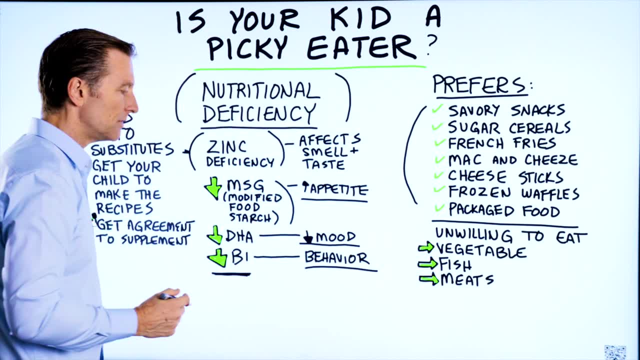 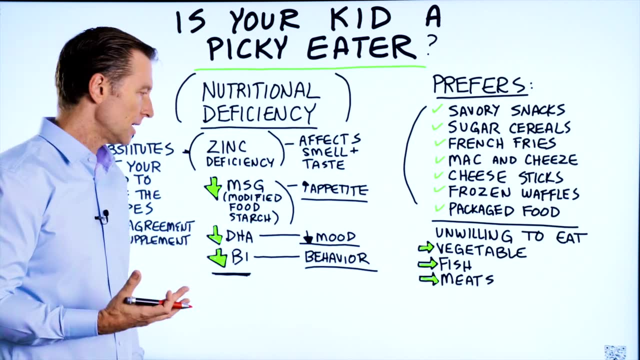 to eat correctly, right DHA can help that greatly. And then we have vitamin B1. If the child is deficient in B1, that also severely affects the behavior as well. So if a child has enough B1, they're going to be calm, They're not going to be restless, They're going to have more self-control. 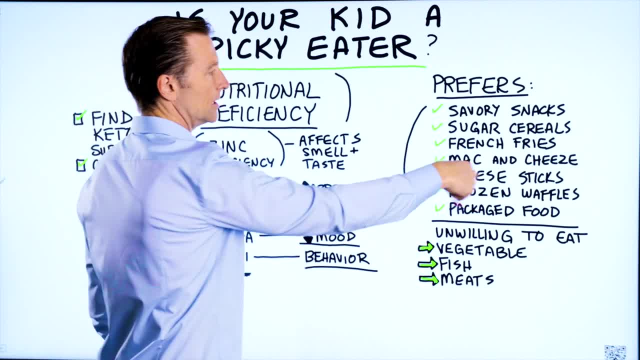 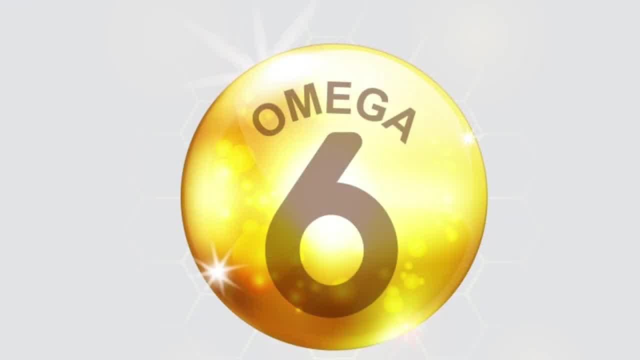 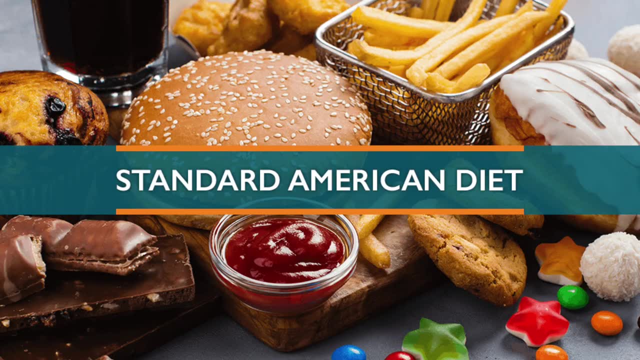 What creates a deficiency here? These foods- right here: refined carbs. What creates a deficiency here? All the omega-6 fatty acids in these foods- right here. If you're unfamiliar with omega-6, I put a link down below. But an average diet is very heavy in omega-6 and very low in omega-3. 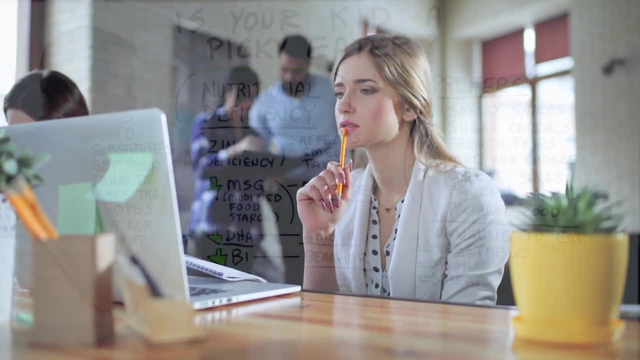 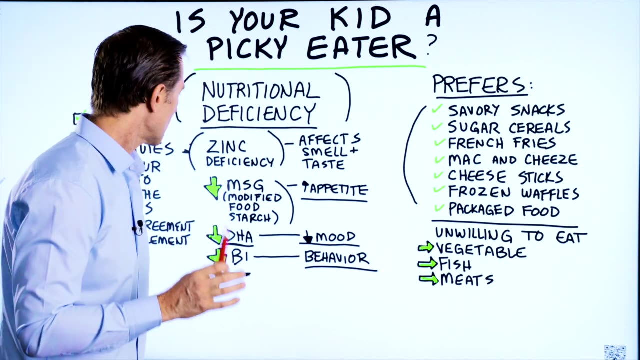 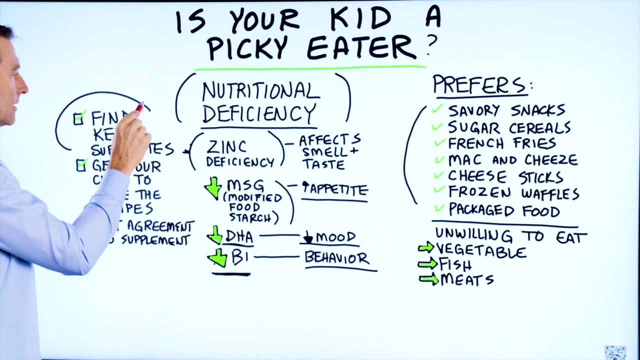 fatty acids. What can you do in addition to giving them some zinc, avoiding MSG as much as possible, adding DHA and B1?? Well, there's a couple of things To make the transition from here to healthier foods. I would start looking at a substitute food, And there's a lot of keto.